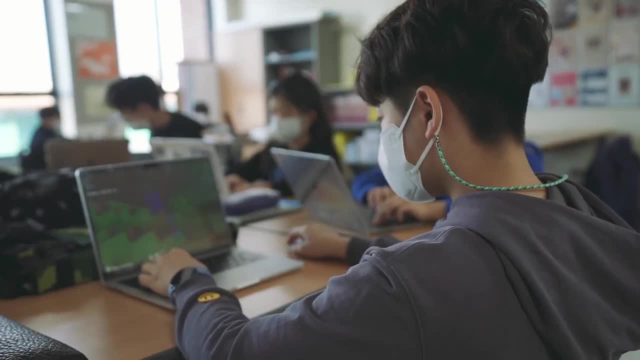 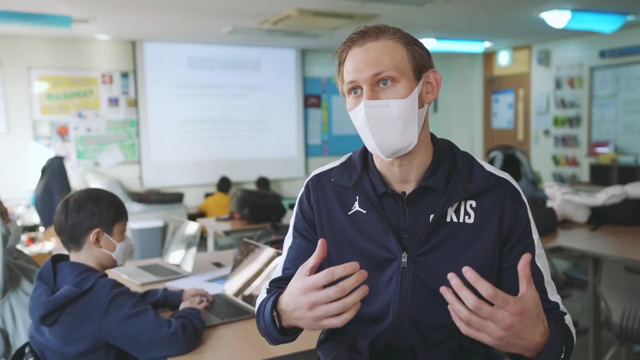 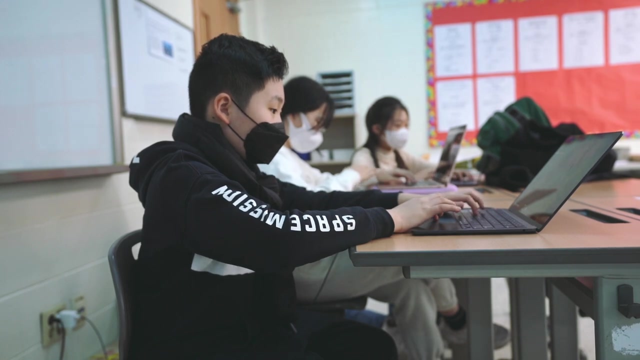 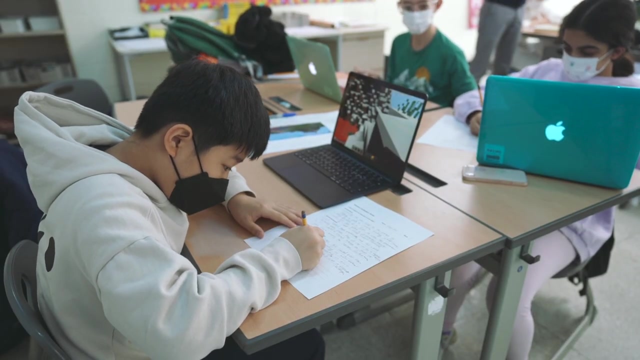 This was our geography unit and we had students learning about how they would depend, adapt and modify the environment to meet their needs. Before we had students enter the Minecraft world, we had groups kind of split up and researched different examples of volcanoes around the world. We practice 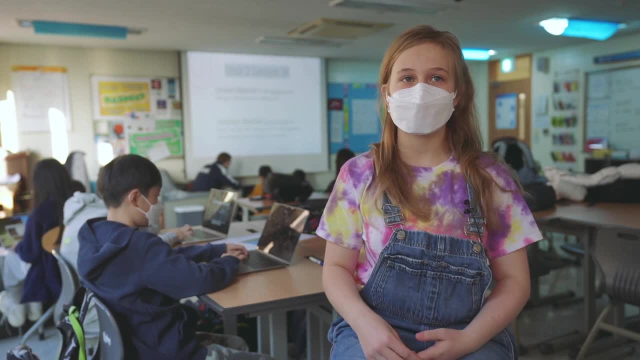 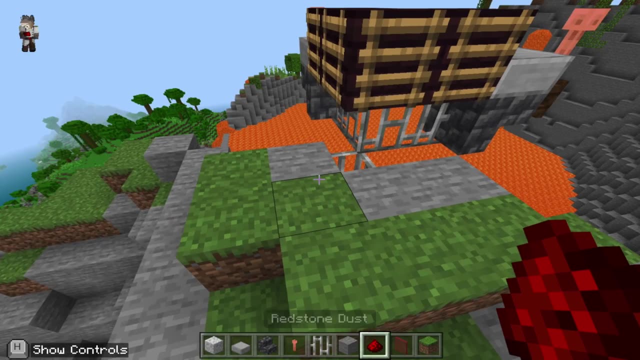 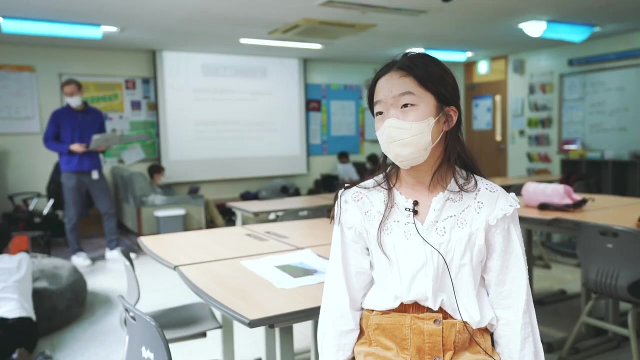 making claims and evidence and reasoning and like researching and like looking at volcanoes and like how they impact humans and civilization In this world, in Minecraft that has a volcano, and we have to create things that show our civilization adapting, modifying and depending on the volcano For modify. we 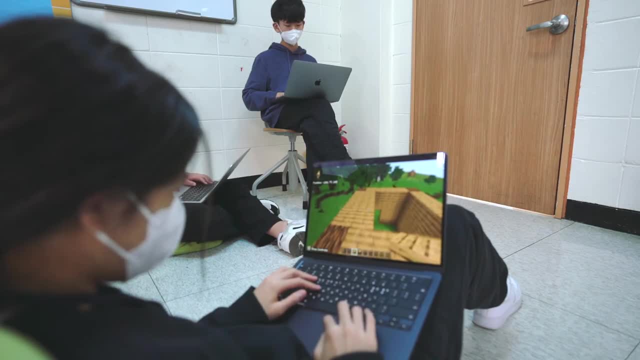 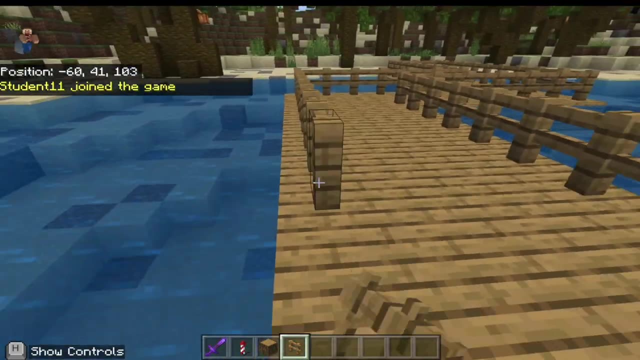 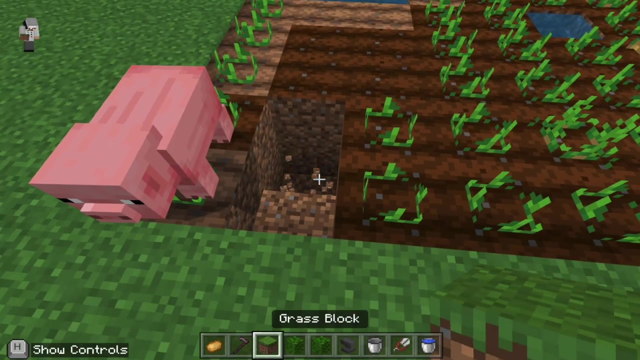 built a like stargazing area. with a telescope, People could look at the stars from a greater height. I am right now working on a bridge that connects, like, each island For depend. we're making a farm because we're like depending on the fertile soil And then adapt, we're. 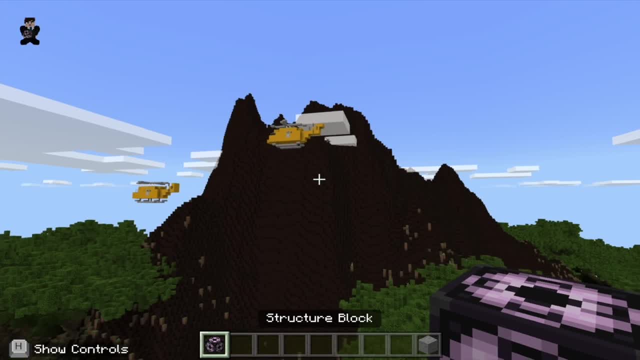 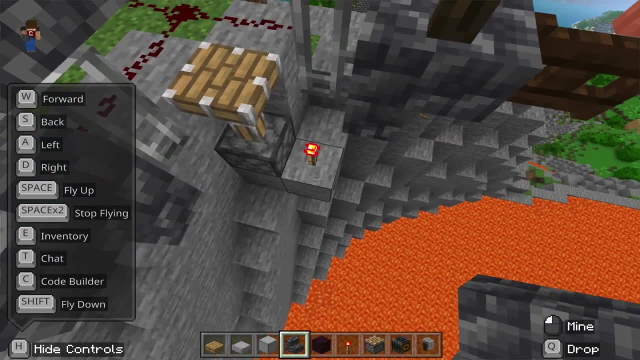 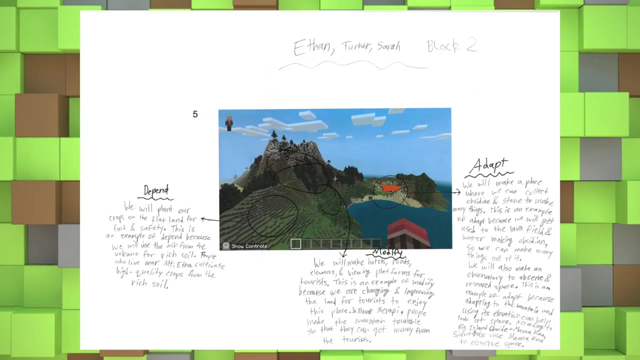 building a helicopter so that way, when the volcano explodes, we have access to the helicopter so we can get out. So what we plan to build like device that could measure the levels of the activity of the volcano. This sheet is pretty much planning out what we will do for each depend, adapt and modify. 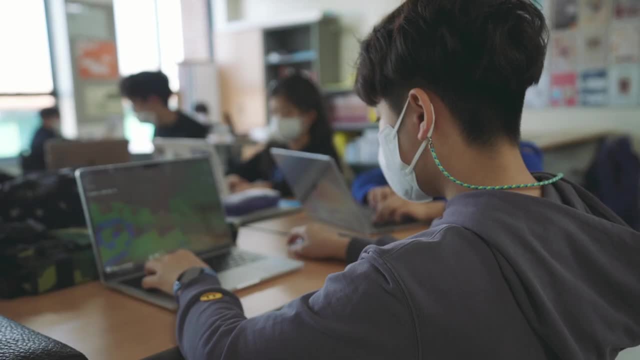 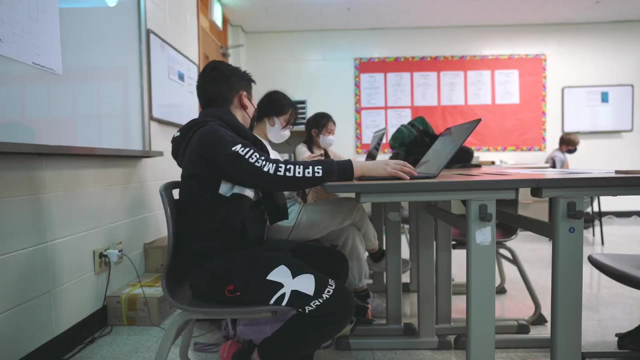 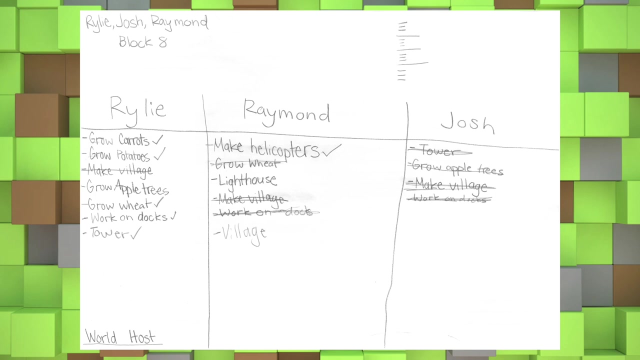 I see a lot of engagement. I think the biggest thing is that all groups are really focused. They're working together. I see great teamwork, great communication. We each assigned ourselves jobs, So, hey, you can work on that, I'll work on this. 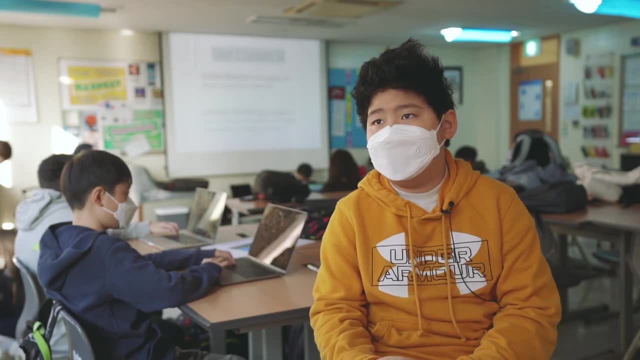 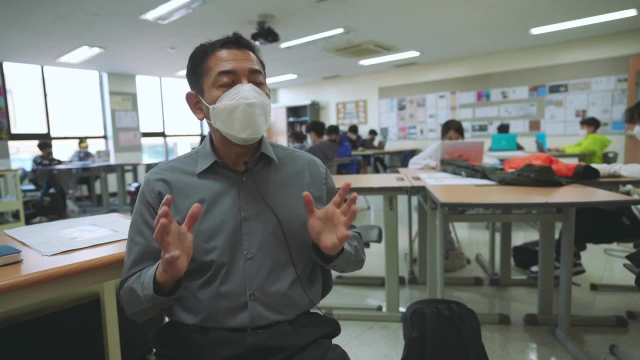 and you can work on that. We all agree, and so we just get on task right away. As soon as we mentioned we're gonna use Minecraft. wow, kids were excited. For the kids it's exciting to have that, but also as teachers when you see that new. 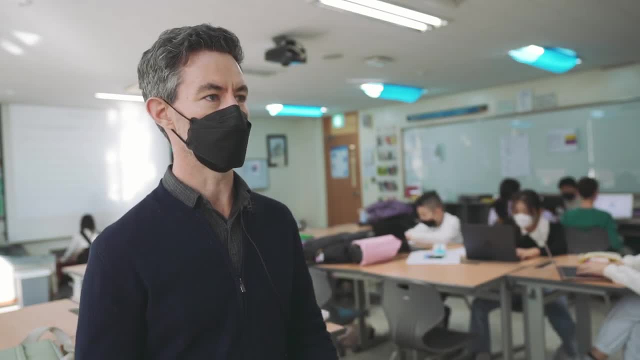 possibility. we also get excited about that kind of learning, So I think it's a really good opportunity for us here at KIS.